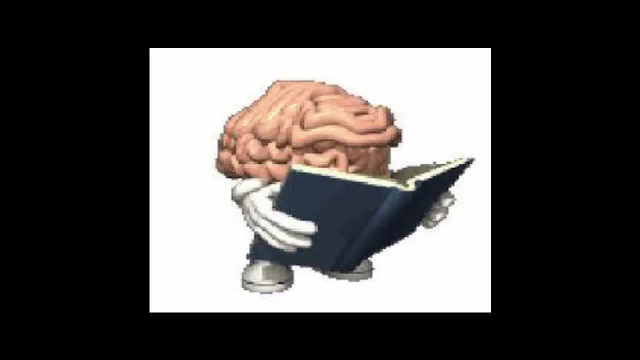 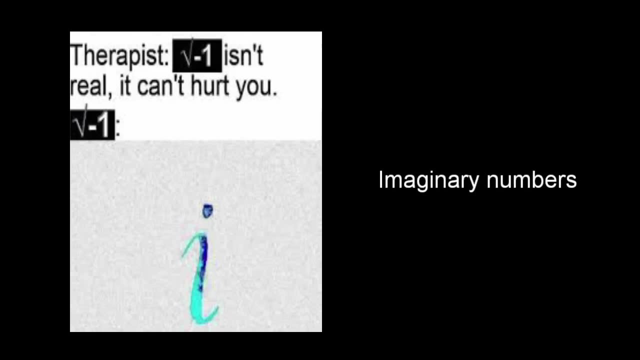 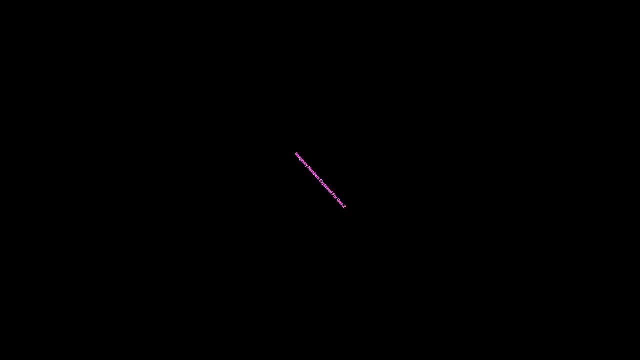 What's popping? Imagination through voice, Imaginary numbers. While they do be dead-ass, no cap, it's kinda wacky. I'mma make it an understandable VR with the use of gen z slang: The Ohio numbers. what are they made of? 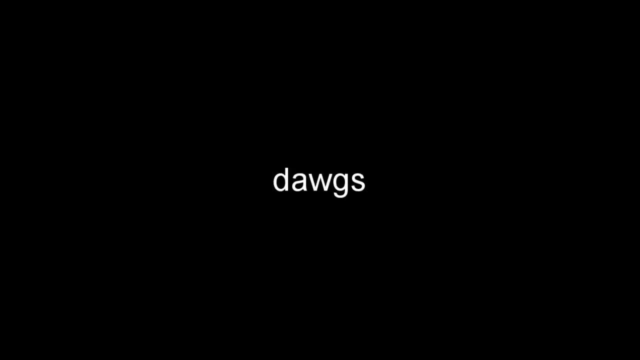 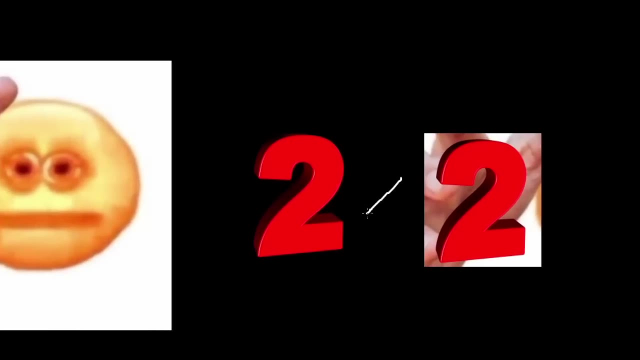 To find that out, we're going to take a quick look at square numbers. These dogs are the light-skinned starers of basic math. To find a perfect square, take any number and dupe it, and then multiply them together. There's your perfect square. 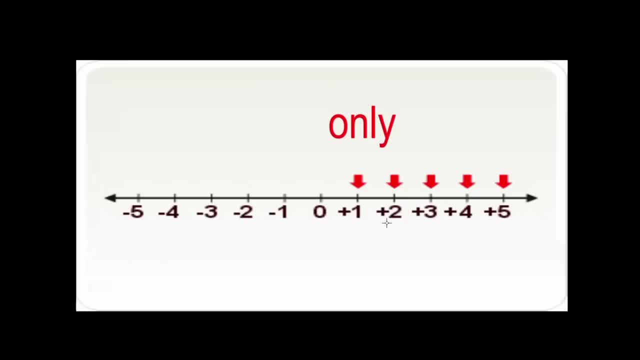 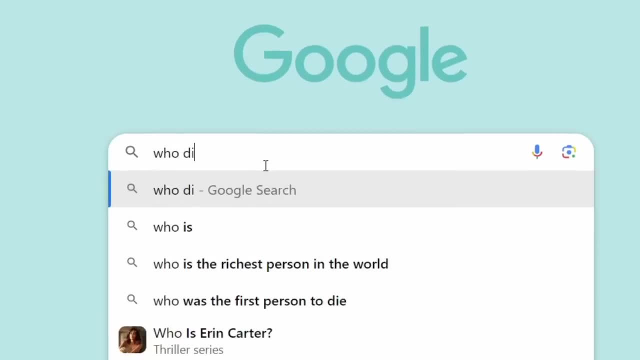 You can do the same with negatives. however, you may have noticed that only positive integers are moving. At no point do you get a negative number as the output. So around 1545,. some Rizzler called Joelomo Cardano called around on TikTok in search. 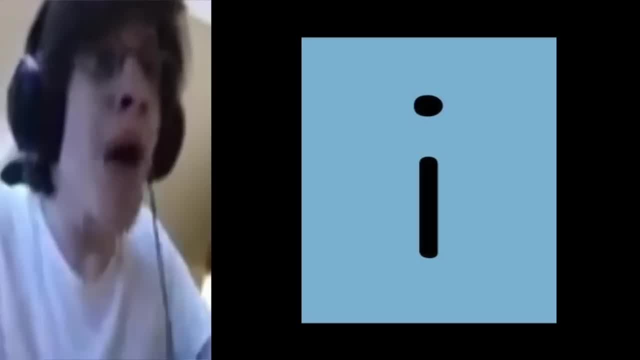 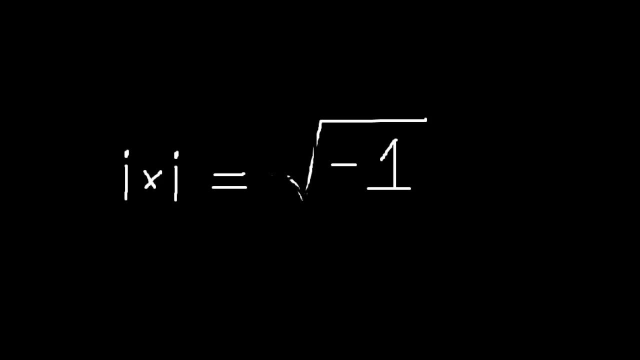 of Lux Maxxing Clothes, And that's when he came up with R, The imaginary unit. I is the square root of negative one, which pretty much means that when you multiply I by itself, you get negative one On guard. this may come across as a cap. 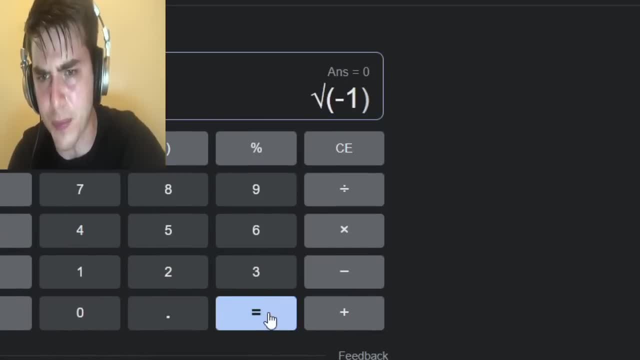 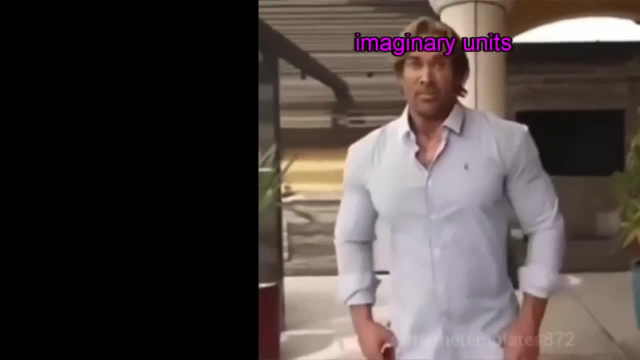 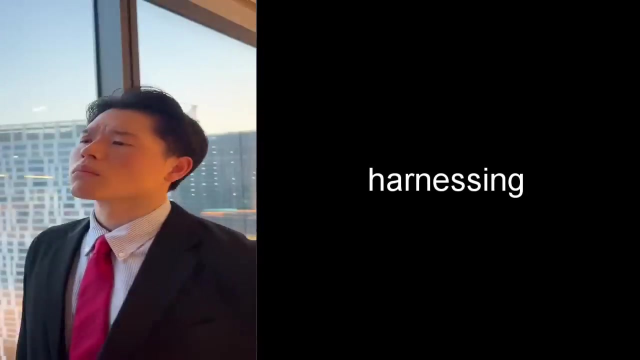 When you try to square root negative one on a normal calculator it'll spit you out. Pay down bad respect. But just hear me out, pal. Imaginary units are built different, So let's put on our thinking caps and by harnessing 200 IQ, Level 3- Yet Ohio Gods, we 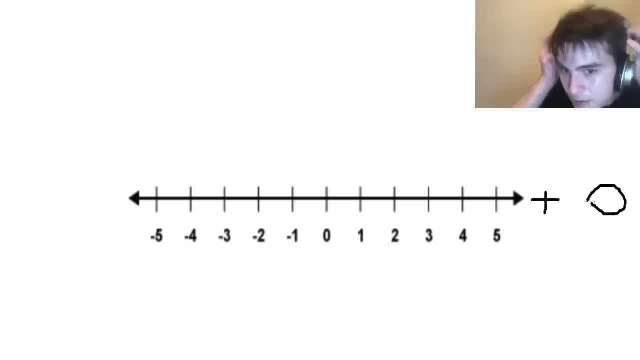 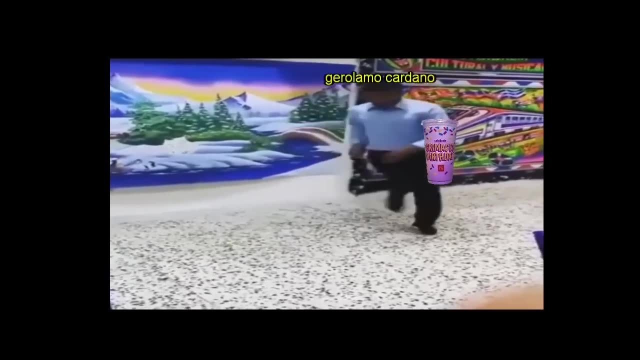 get the number line. What the actual frack am I saying? The number line, The real line. It contains all of the positive, negative integers, decimal fractions and everything in between. Now this Cardano guy went and took a sip of the Grimace Shake and cranked some 90s and 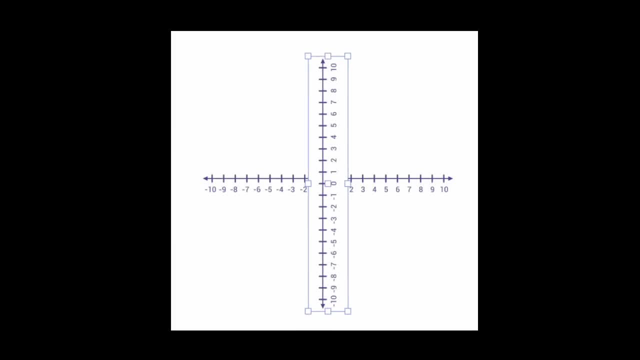 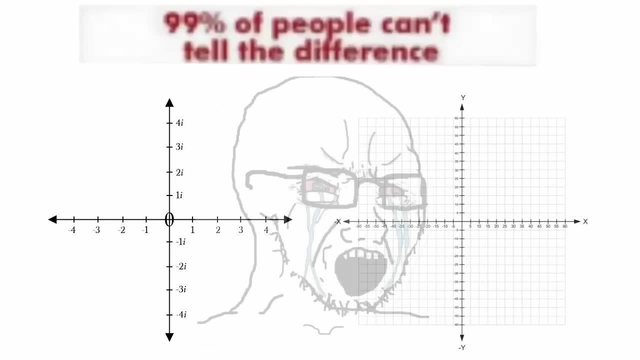 like, literally rotated the real line by 90 degrees And bam, The imaginary number line. Now let's play a quick spot, the difference game here. 99% can't see it, and that's because there pretty much is no difference. Let's call the imaginary rail grid thingy the complex plane. 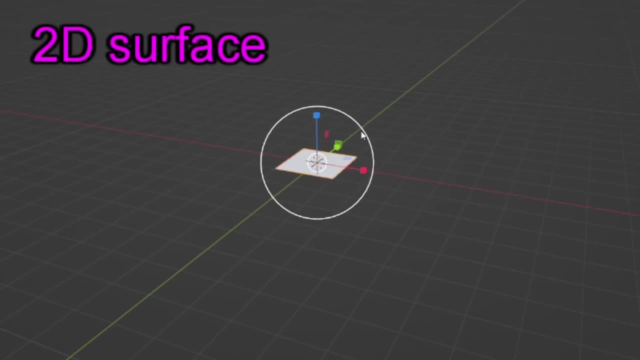 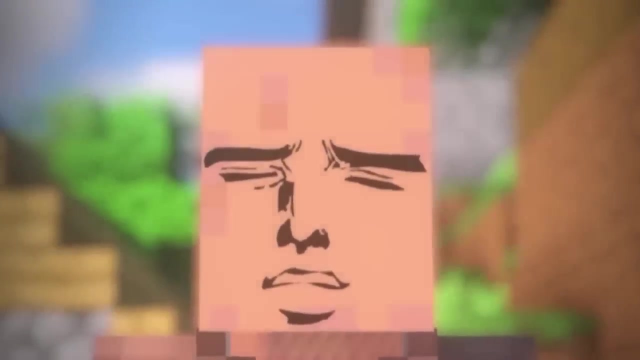 And no, It's not a goofy R plane. It's referring to a 2D surface that expands indefinitely in all directions Like a Minecraft flat world, Except without the villagers. So the complex plane and the Cartesian plane pretty much describe the exact same thing. 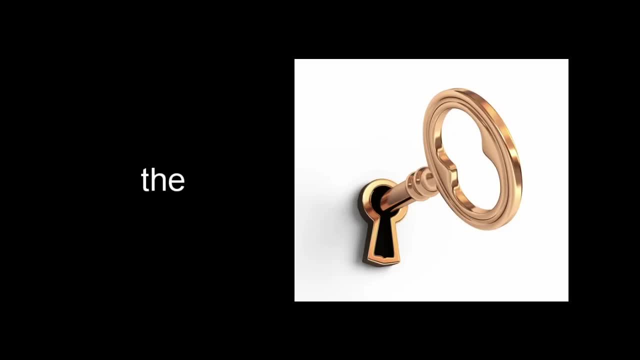 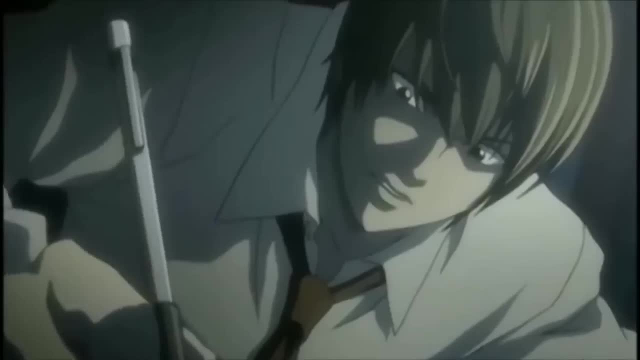 An environment containing X and Y axes in which points can be placed. The key distinction between the two is how the complex numbers perform in game. Their notation is written as simple addition problems like What's 9 plus 10? 21. You stu-. 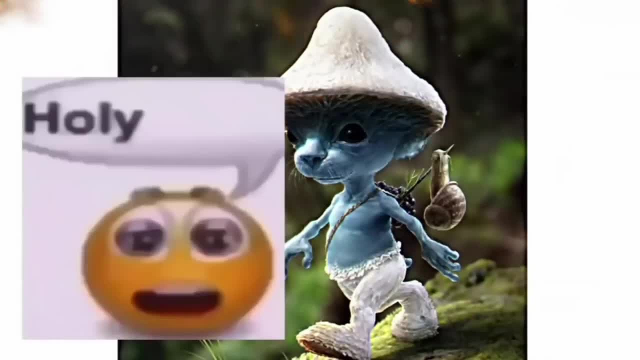 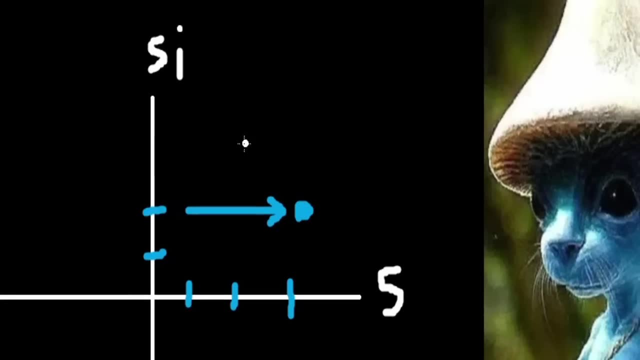 It's a real number being added or subtracted by an imaginary number. So if the smart cat wanted to find the point 3 plus 2i, add 3 across the real axis and add 2 on the imaginary, and bam. 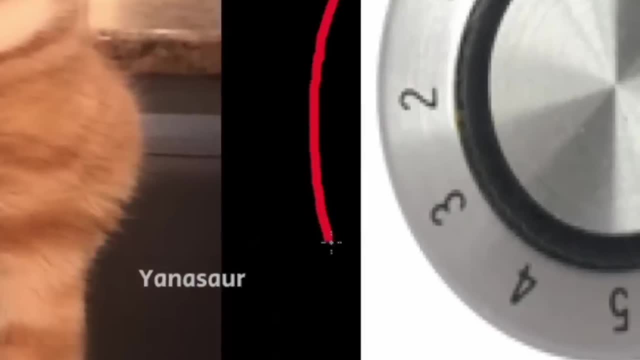 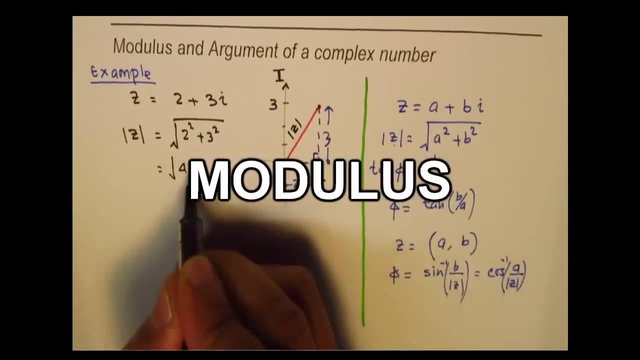 There's your point. Alrighty, now turn your math maxing dial up to 11 out of 10, because now we're gonna have a look at modules. If you wanted to find if a complex number was bigger than another, you can't just do this. 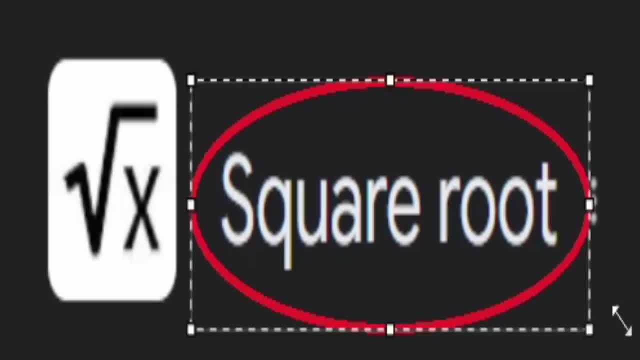 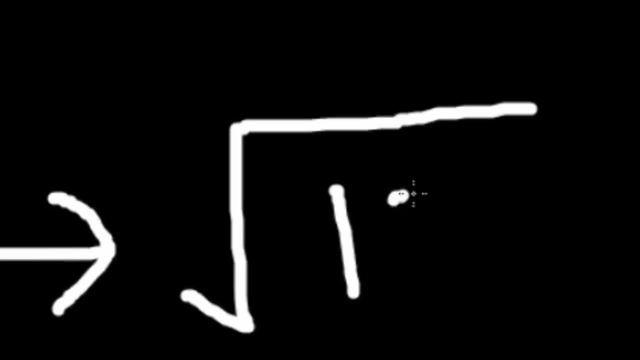 To get them busting, you gotta draw this here, The square root, And inside of it you square the real number and the imaginary number and add them together. Okay, fam, now do the basic arithmetic And there you go. That may have felt like navigating the house after the lobotomy. 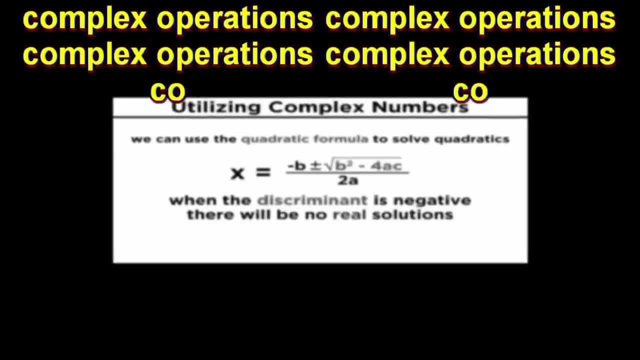 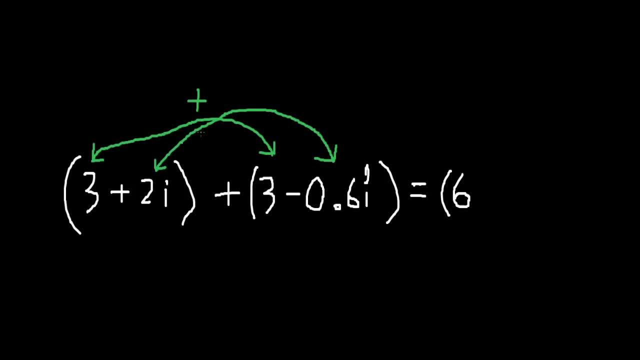 So now we're gonna have a quick yappy session about complex operations. To add, you simply add the two real numbers first, And then flowberry fizz, the imaginary ones too, And there's your sum. And for subtraction, it's legit the same but with minus. 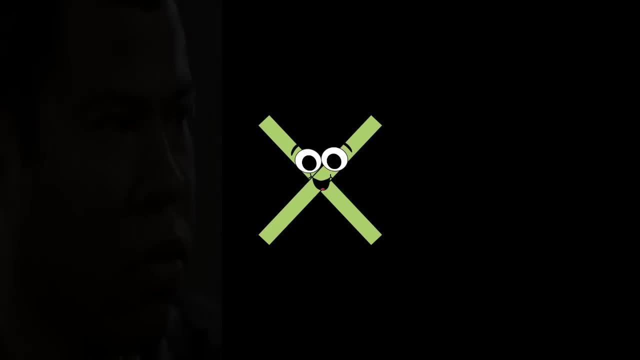 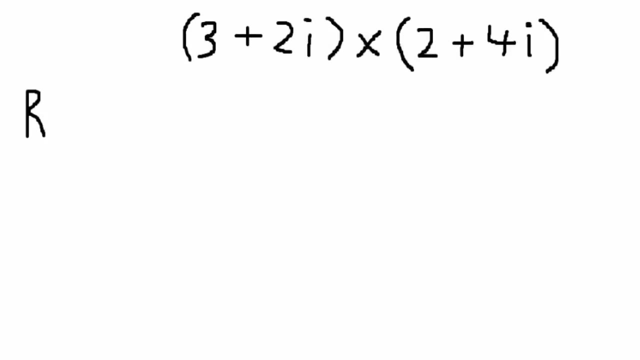 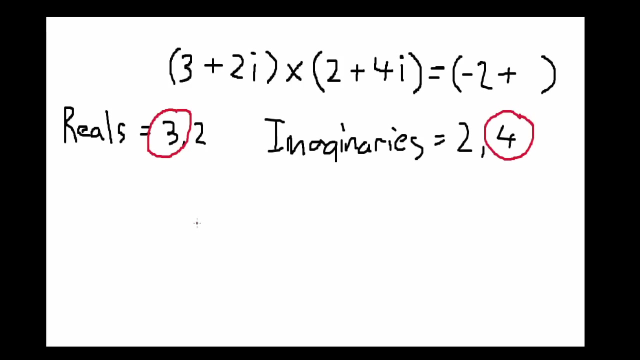 But. But Multiplication and division is like a little bit harder. You can follow this formula: The real numbers multiplied minus the imaginary numbers multiplied is the new real number And the first real number multiplied by the second imaginary number plus the second real 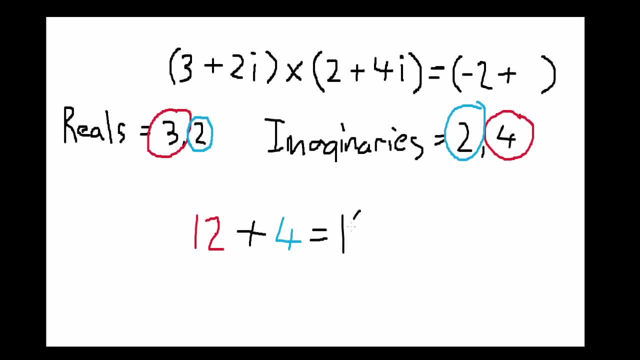 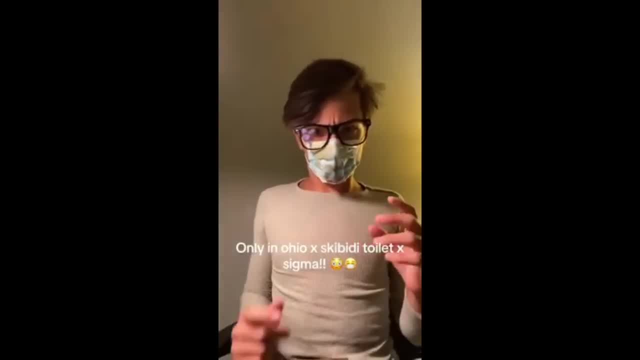 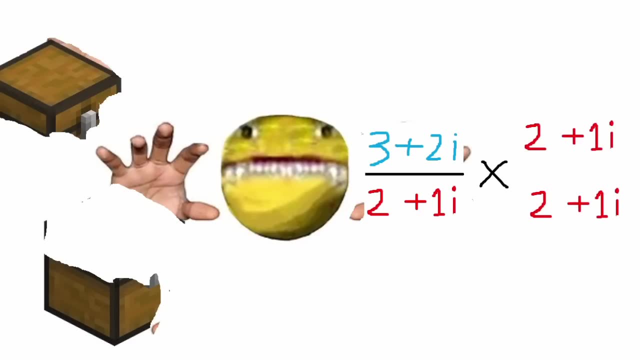 number multiplied by the first imaginary number Is the new imaginary. Only an Ohio complex number, Only an Ohio complex number. Okay, so the division's even worse. What you gotta? get your fraction And multiply it by the conjugate of the denominator. 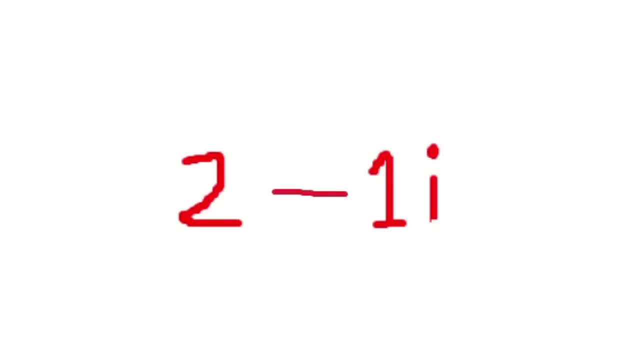 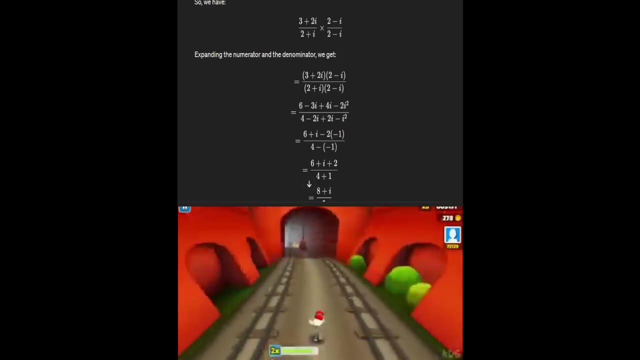 What? Okay, so it's that, but the sign is float. That's the conjugate. So, And you simplify that expression, You break it up to the real part and the imaginary part. That's correct. Thanks for watching this. Khan Academy lesson. 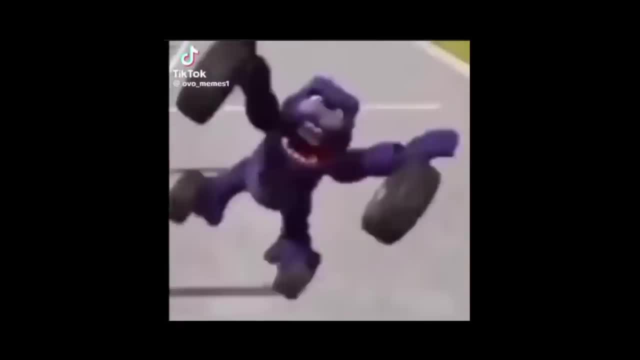 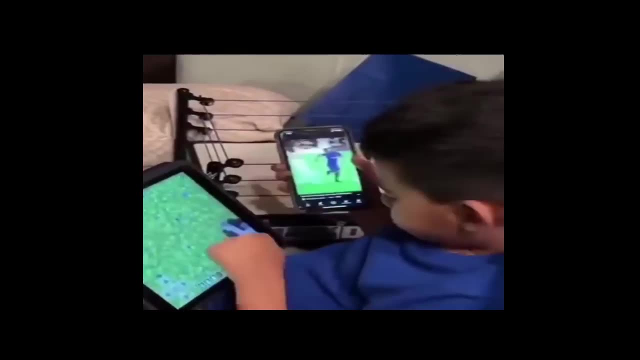 But now we're gonna move on to stuff you only experience at 3am in FNAF bruh Or in a mathematical programming class. The manual box set A thing that looks like something an iPad kid would draw is a backroom's entity looking. 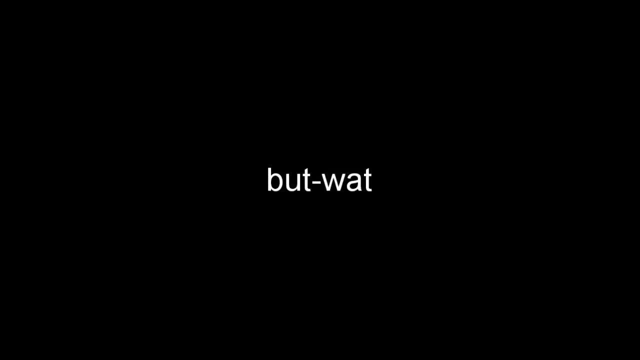 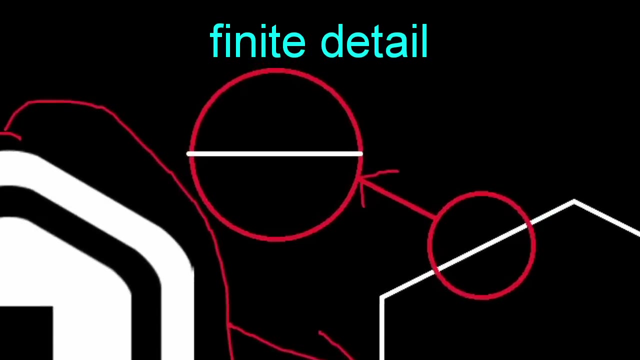 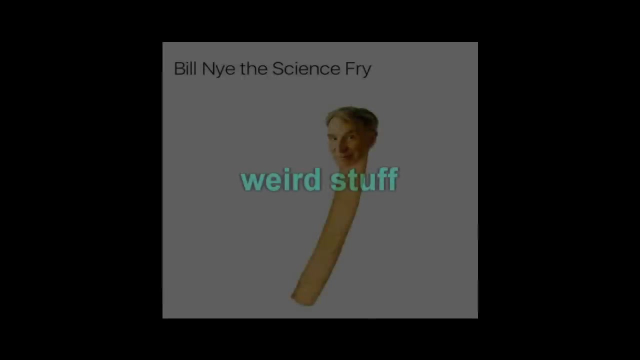 fractal That is generated from this math right here, Okay, but what is a fractal? Take Robux, for instance. The hexagon has finite detail around the edge. The difference is that this geometry has infinite details. Therefore, when you generate the manual box set, you get weird stuff like itself and: 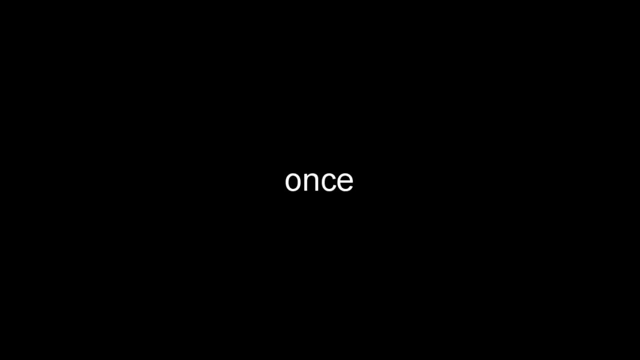 itself. That's crazy, And I was crazy once They locked me in a room. I robbed a room. I robbed a room with rats, And rats make me crazy, Crazy. I was crazy once They locked me in a room. 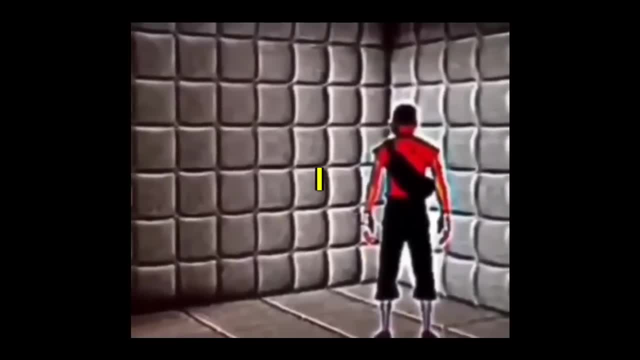 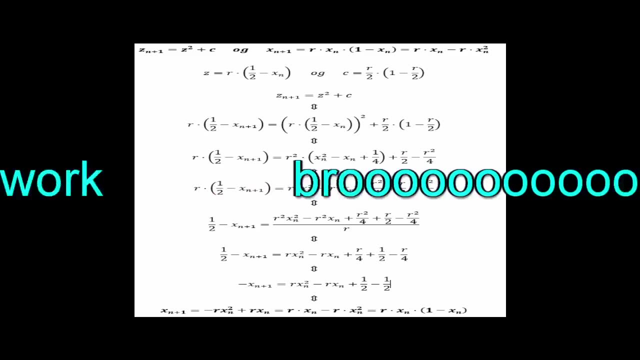 I robbed a room. I robbed a room with rats, And rats make me crazy, Crazy, I-. So when you run this equation in a computer program, it generates this fractal. But how does the math work, bro? Z starts at zero. 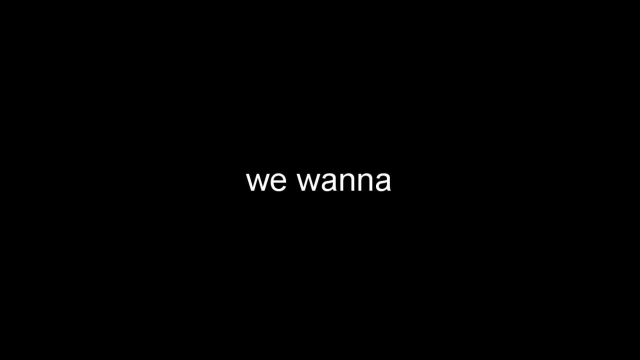 And for every point in time it's zero. And for every point in this area we want to check. What are we checking? As, if the modulus exceeds two, If it does, its a suscy buca. If it is a suscy buca, let the educated sit down and think for a second. he is free. 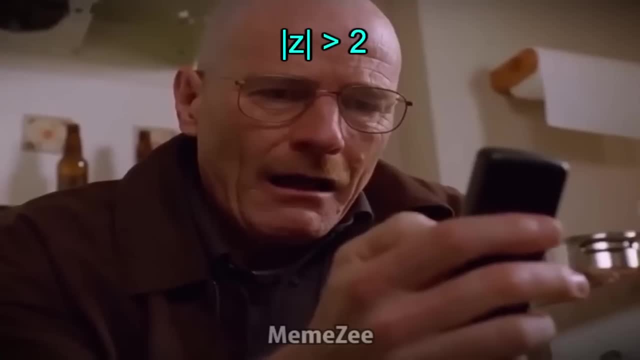 And this kid named Finger didn't go into the set. And no warning, No warning. Somebody says that you killed Tetris out of nowhere. We are iterating the function In sigma-mail terms. we are multiplying our muons-streak by itself and then adding our 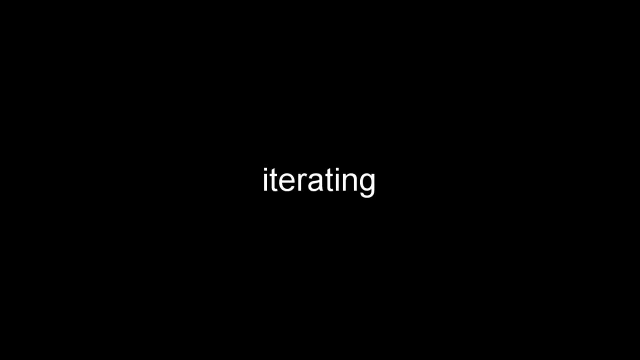 res, Our res is a complex number. It is and it represents a given point. If the discord mod of Z reaches above 2, after iterating a bunch of staples, the eyes will not be Land, And if Z reaches above 2.. 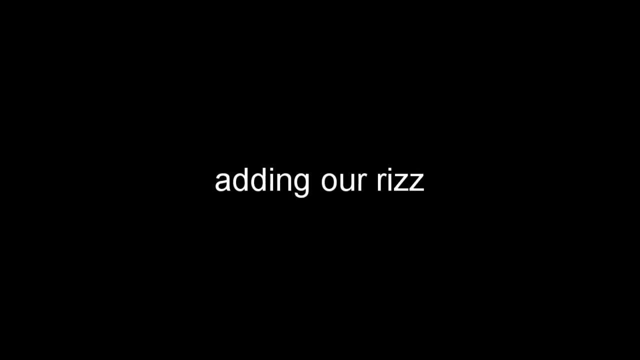 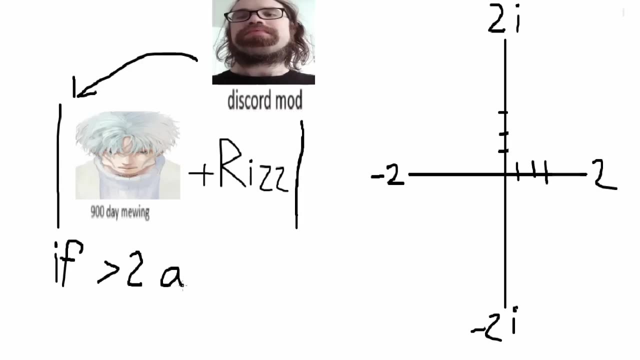 Then you left without even handling the card streak by itself and then adding our Riz. Our Riz is a complex number and it represents a given point. If the Discord mod of Zed reaches above 2 after iterating a bunch, it doesn't deserve. 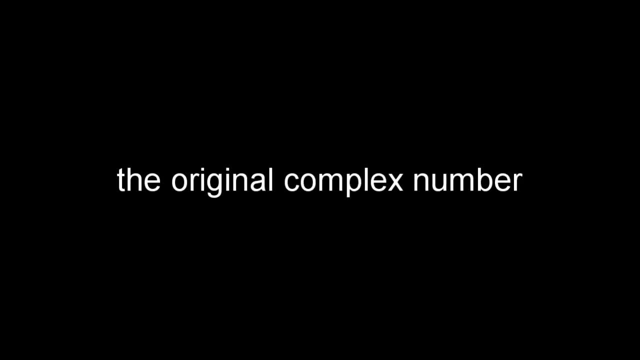 iSpice. but if it stays under 2, the original complex number gets mapped to the complex plane. So it does this for every point that it can and you get that It's pretty wild. So we've talked about the Quandel Dingle numbers and what they are and what they represent. We've